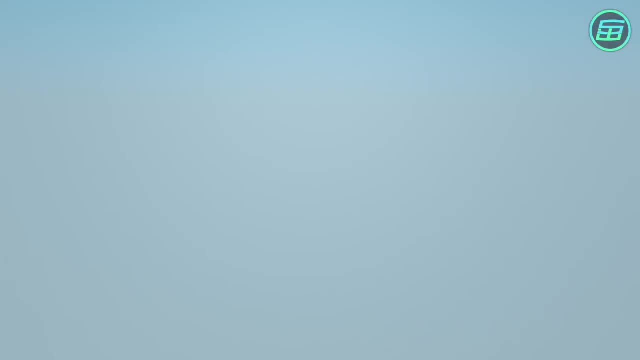 If water contains high amounts of calcium and magnesium ions, it's considered to be hard water. Some other metal ions, such as those of aluminum, barium, iron, manganese, strontium and zinc, also contribute to the hardness of water. 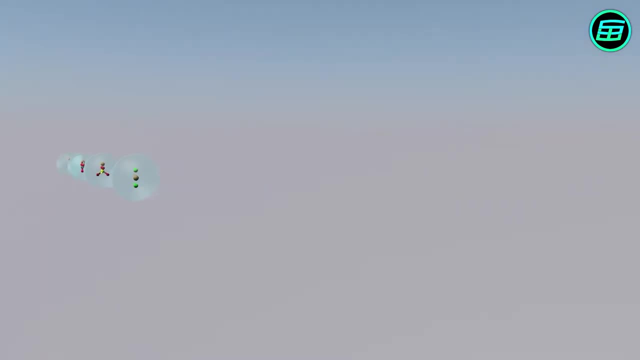 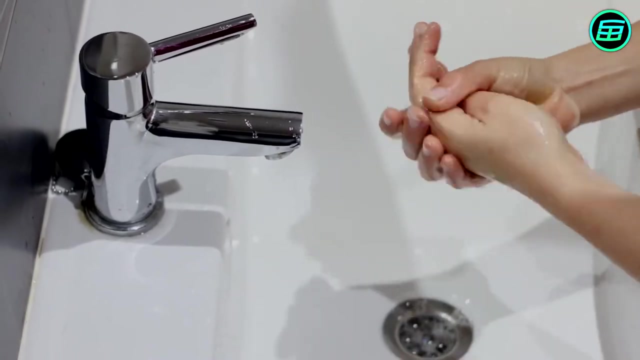 These ions are found in water in the form of carbonates, bicarbonates, sulfates and chlorides. Another way to tell if water is hard is if it doesn't form lather. well, This failure to lather is due to the relationship between the two ions. 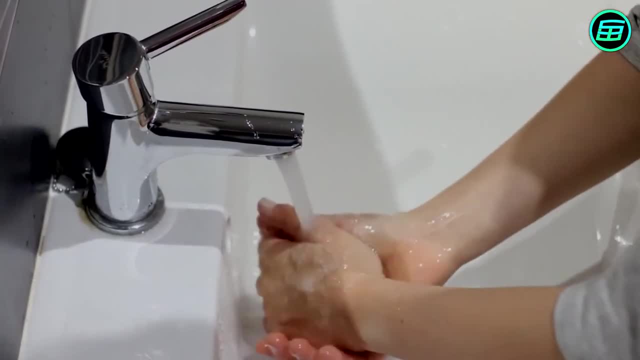 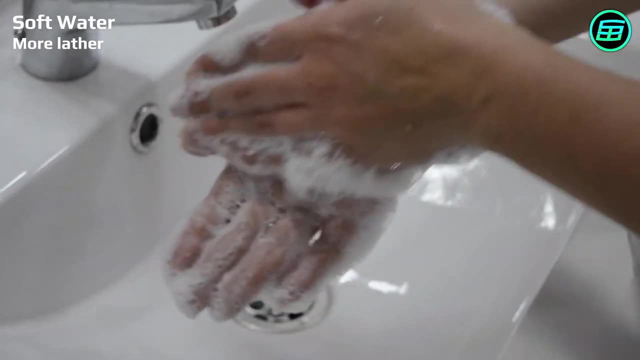 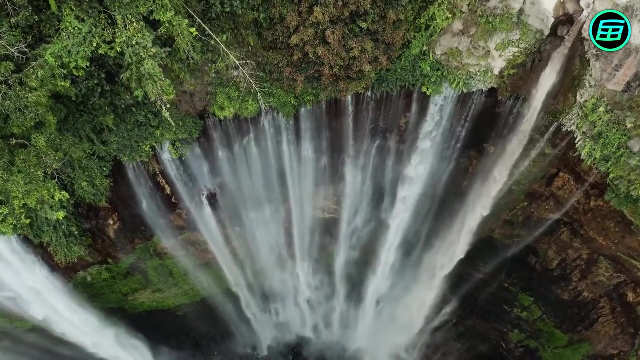 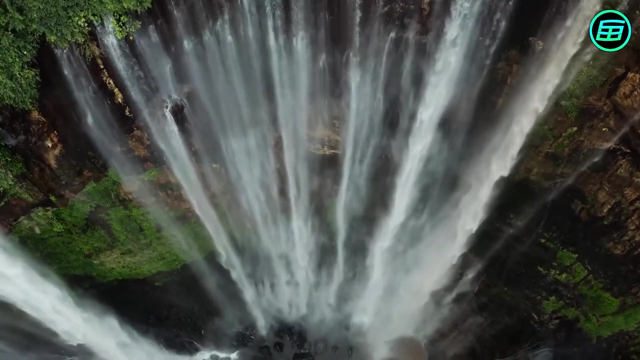 There is a reaction between calcium and magnesium ions and soap molecules. The resulting molecules are insoluble in water and remain at the surface. Less soap molecules means less lather. When rain falls to earth, it percolates underground During this process. if rainwater comes across deposits of limestone, chalk or gypsum. 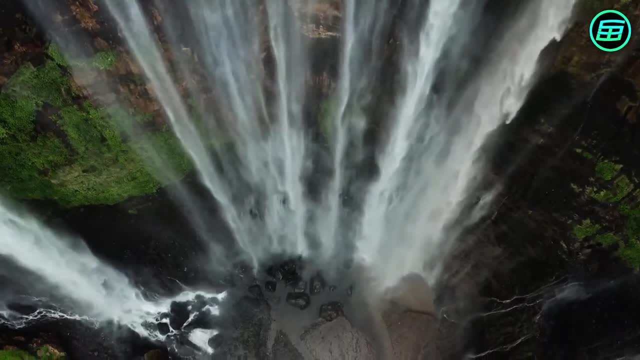 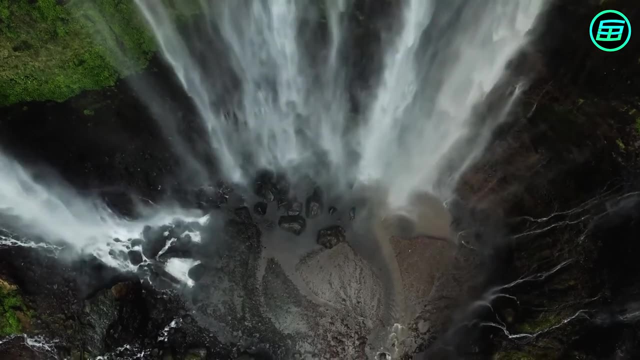 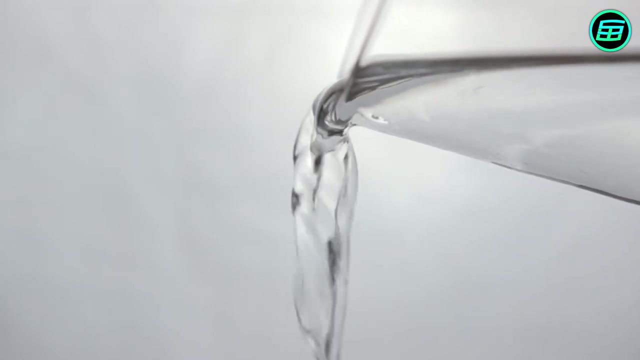 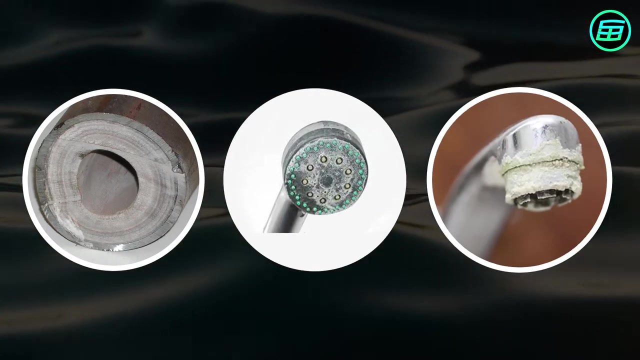 which are made up largely of calcium and magnesium. these metal compounds pass into the water, causing it to become hard. Hard water is generally not a health risk, but it is a nuisance. When hard water is heated, a certain amount of water evaporates, causing the minerals suspended in it to precipitate. 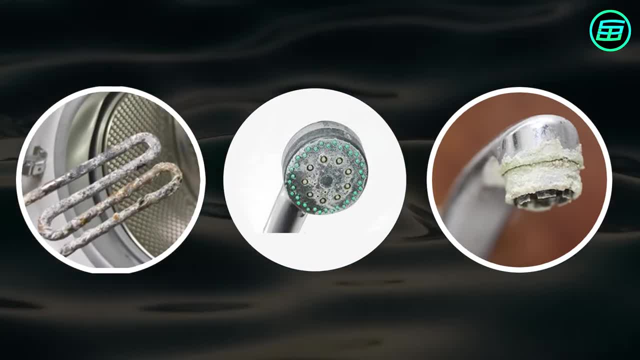 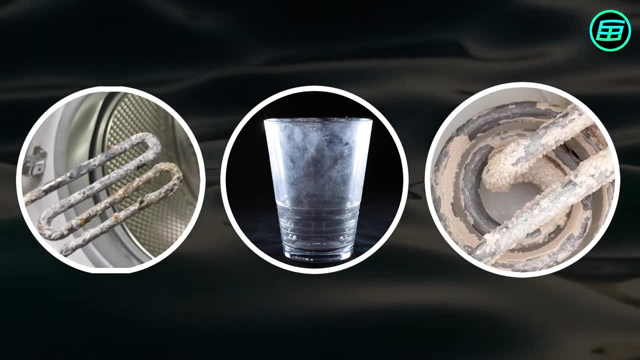 These residues can then accumulate inside pipes, water heaters, washing machines and dishwashers. The result is reduced to a high concentration. The result is reduced to a high concentration. The result is reduced to a high concentration. This causes reduced water flow or blockages. 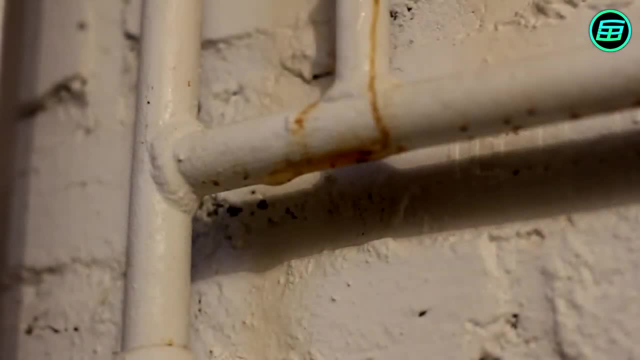 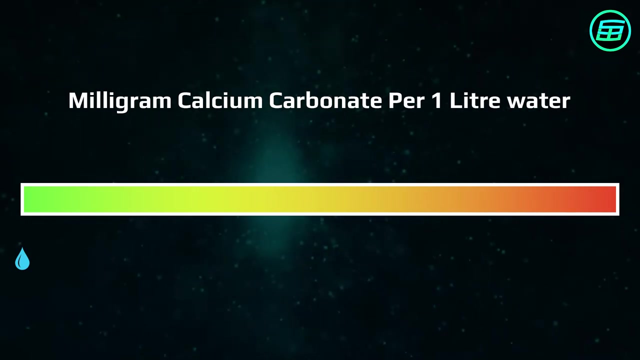 stress on pipes and fixtures, spots on glasses and dishes cleaned in a dishwasher, and less effective clothes-washing due to a lack of suds. According to the World Health Organization, water containing calcium carbonate at concentrations below 60mg per liter is generally considered to be soft. 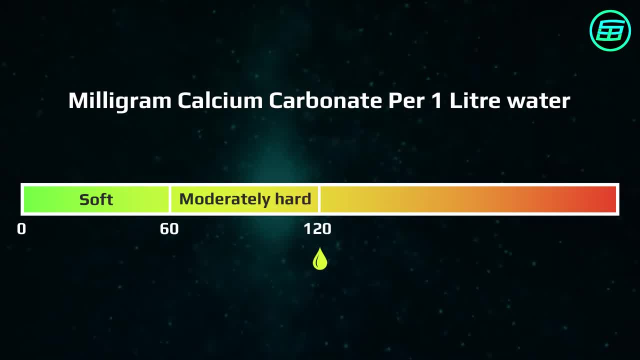 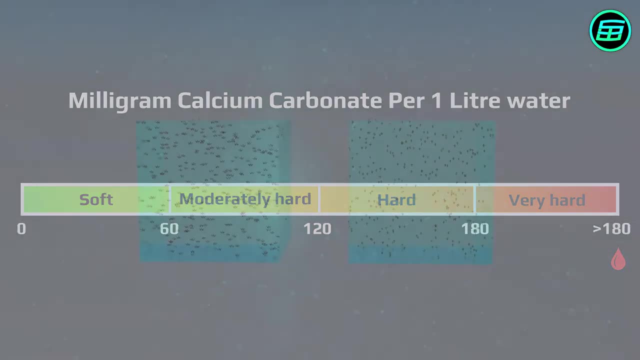 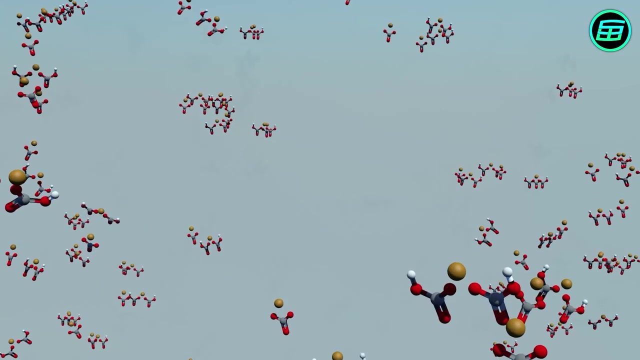 60-120mg per liter. liter is moderately hard. 120 to 180 milligrams per liter is hard and water with more than 180 milligrams per liter of calcium carbonate is very hard. water hardness caused by the presence of just calcium and magnesium carbonates and bicarbonates is called temporary hardness and can be removed. 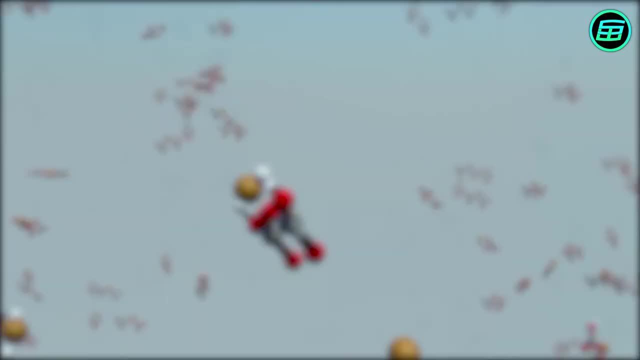 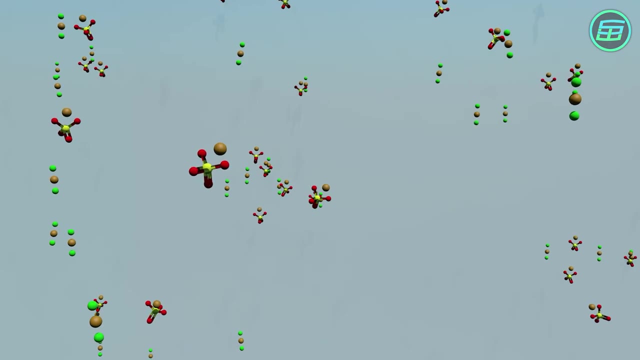 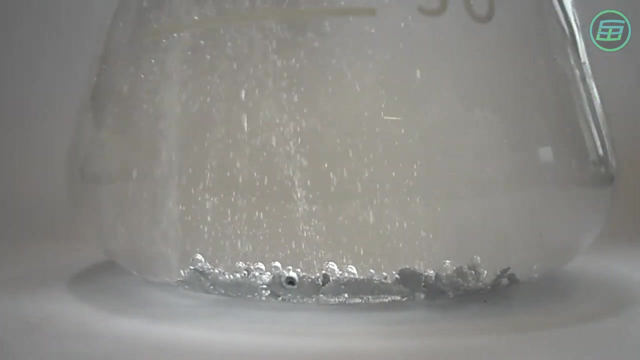 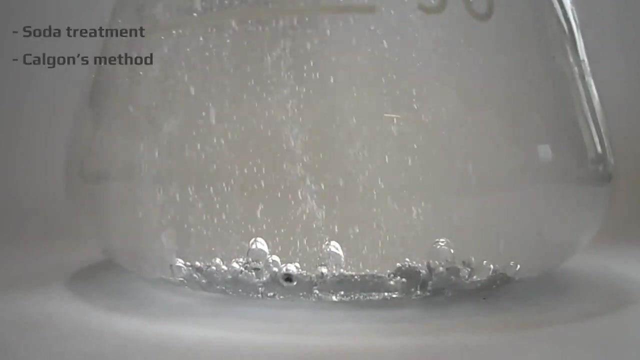 by boiling the water and then filtering it. on the other hand, if water hardness is due to the presence of calcium and magnesium sulfates and chlorides, it's known as permanent hardness and can't be eliminated by boiling. removing permanent hardness requires special chemical methods, such as soda treatment, kalgen's method, ion exchange or the resin method. so you. 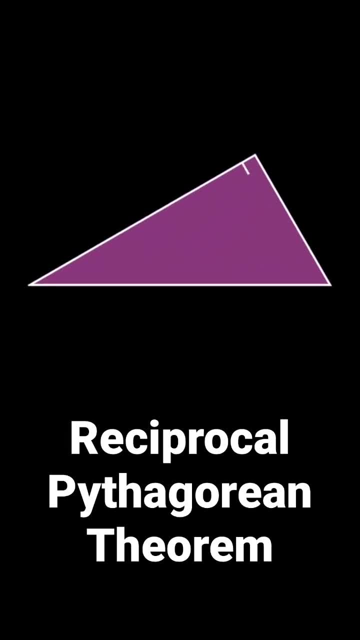 Here's a surprising fact about right triangles you might not have seen before. Imagine you have a right triangle with sides of length a and b and a hypotenuse of length c. The area of this triangle is equal to one half a times b, but it's also equal to one half c times. 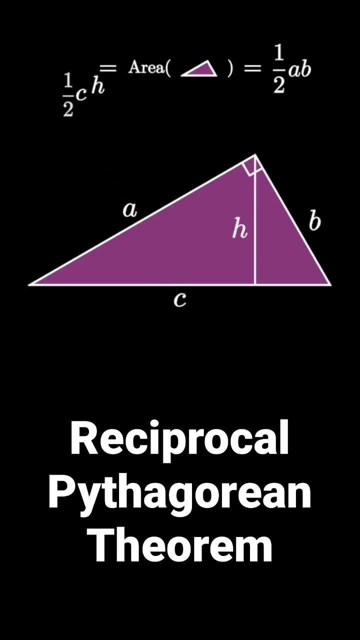 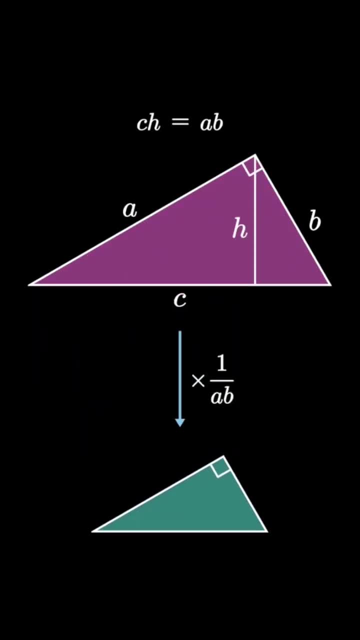 h, where h is an altitude that's drawn perpendicular to the hypotenuse c. This means that c times h equals a times b. Now we scale the right triangle by the quantity 1 over a times b, which produces a right triangle with side lengths of a over a times b, b over a times b and a hypotenuse of c. 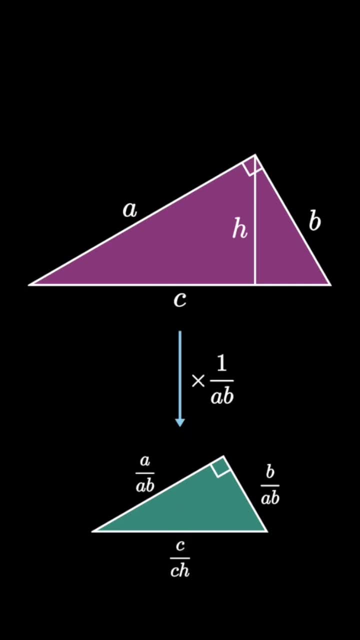 over a times b And ch equals ab. so the hypotenuse is c divided by ch. Notice that the a's cancel in the first side length, the b's cancel in the second side length and the c's cancel in the hypotenuse length. So this right triangle has side lengths 1 over b and 1 over a and a hypotenuse of. 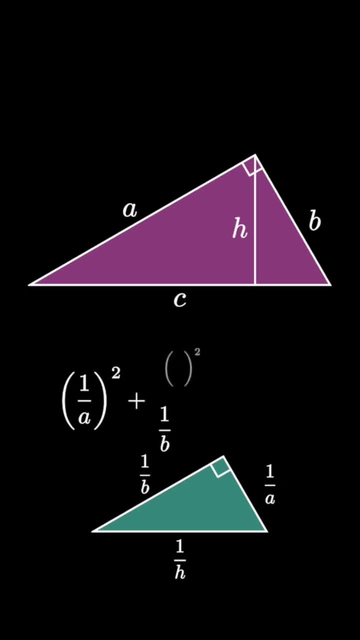 length 1 over h. Because this is a right triangle, we conclude that 1 over a squared plus 1 over b squared is equal to 1 over h squared. So the sum of the squares of the reciprocals of the side lengths in a right triangle equals the square of the reciprocal of the height. 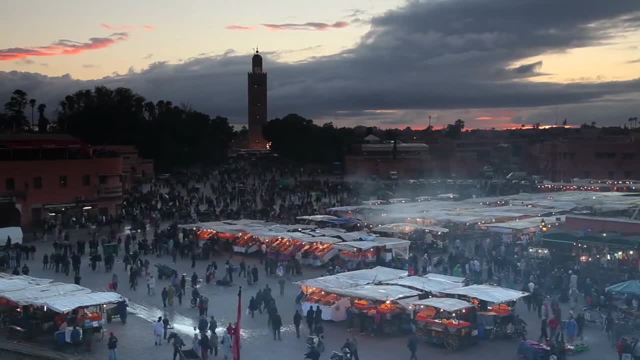 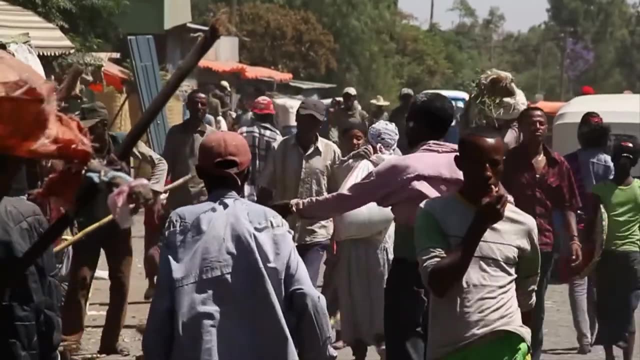 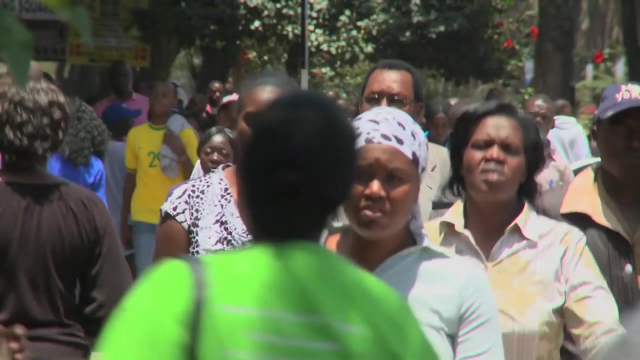 Algeria is the largest country by land area and by population. Nigeria is the largest. Africa has the second largest population in the world, with an estimated 1 billion inhabitants. This constitutes almost 15% of the world's population. Over 1,000 official languages are spoken across the African continent and the largest religious